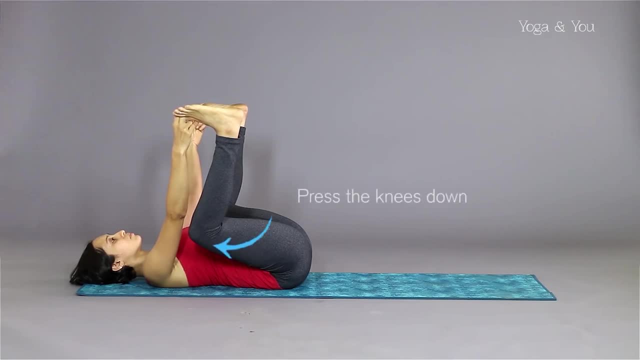 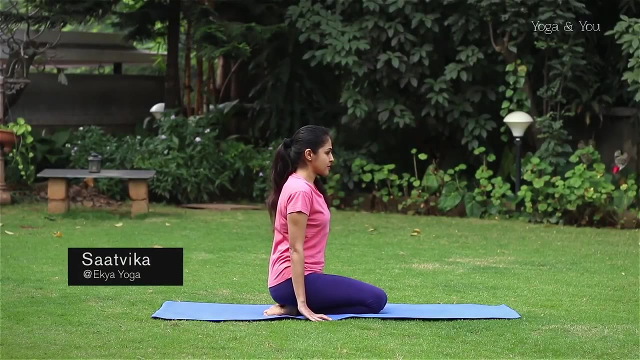 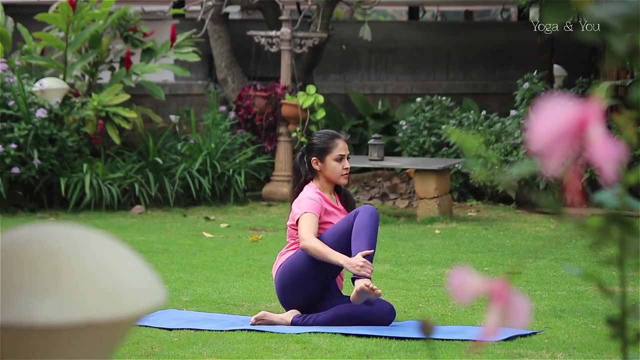 floor. Press the knees down to the floor. Sit in vajrasana From here. lift your hips up and sit to the left. Take your right foot across your left knee and place it on the mat. Make sure your hip does not lift off. 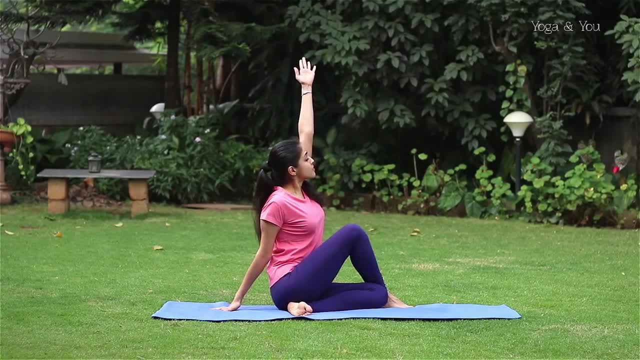 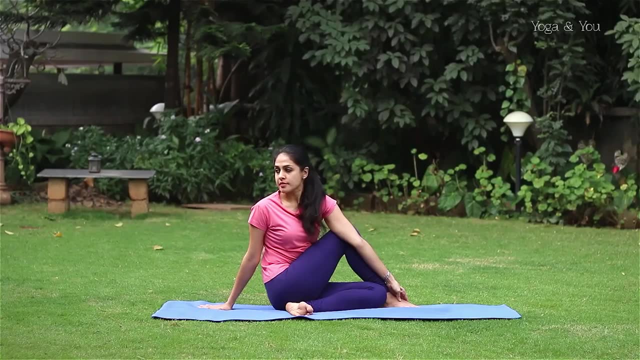 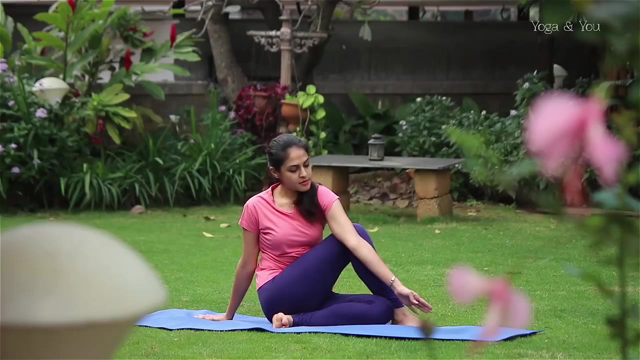 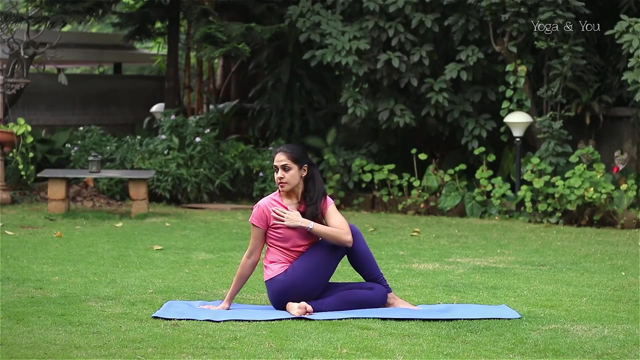 the mat. Place your right hand behind you for support. Inhale, lift the left arm, twist and place your hand on the foot. Look over your right shoulder. If you cannot reach your foot, bend your elbow and place your hand on your shoulder across. Use your upper arm to push the knee back. Make sure. 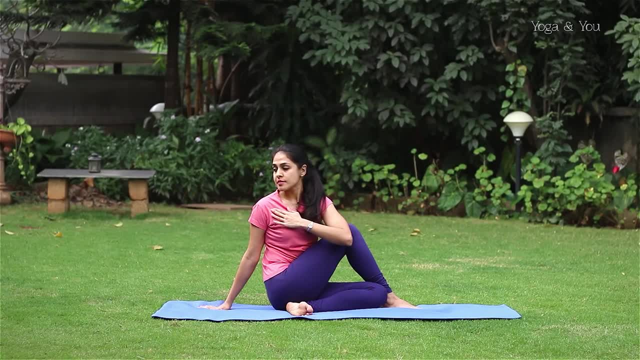 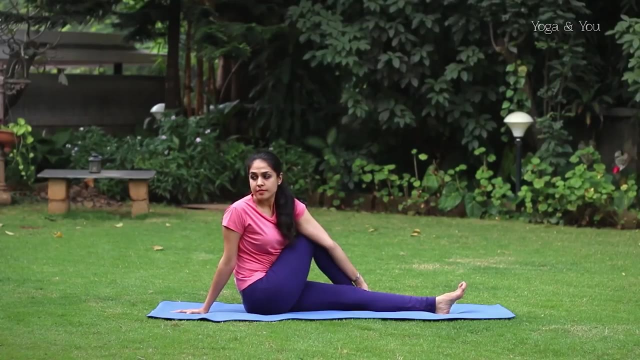 there is no tension in the shoulders To release: Inhale, lift the left arm up, Exhale, bring it down. Release the legs. come back to Vajrasana. Repeat on the opposite side. An easier adaptation of Ardha Matsyendrasana. 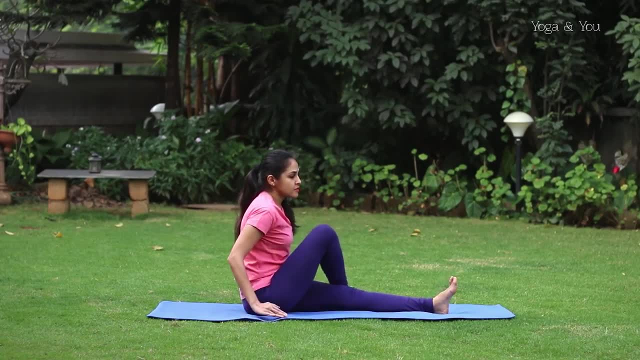 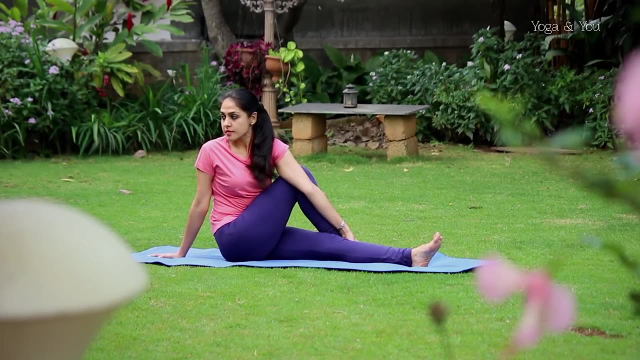 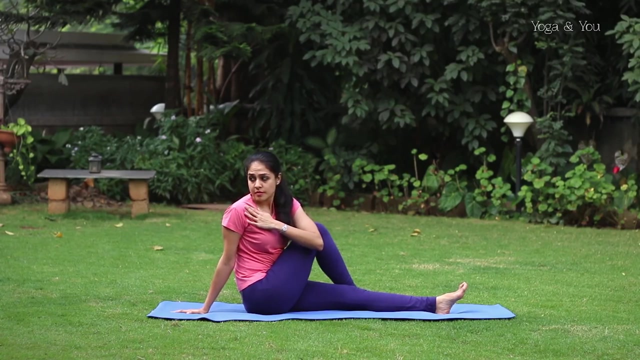 From Dandasana. place your right foot across the left knee, right hand behind you, Inhale, left arm up, twist. place your left hand on the right foot. Alternatively, bend the left hand and place the hand on the shoulder across. Look over your right shoulder To release. 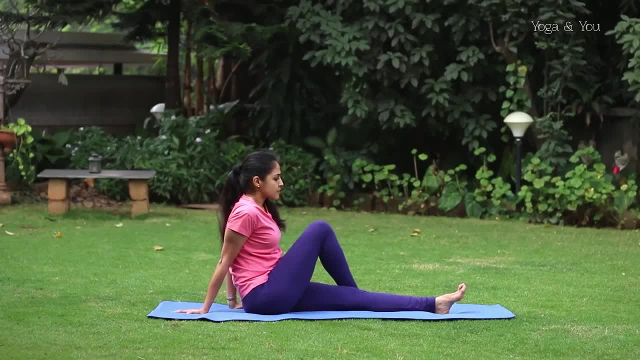 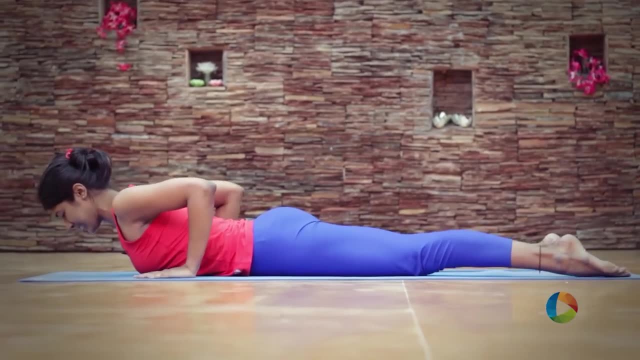 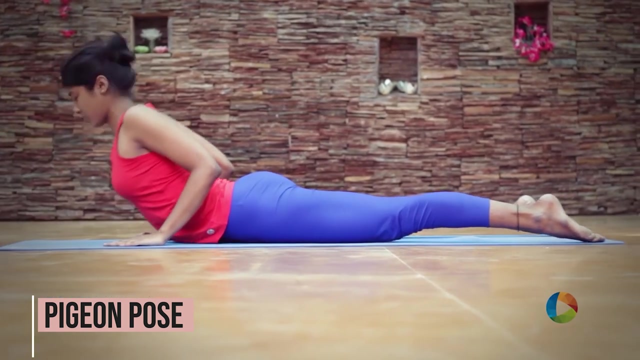 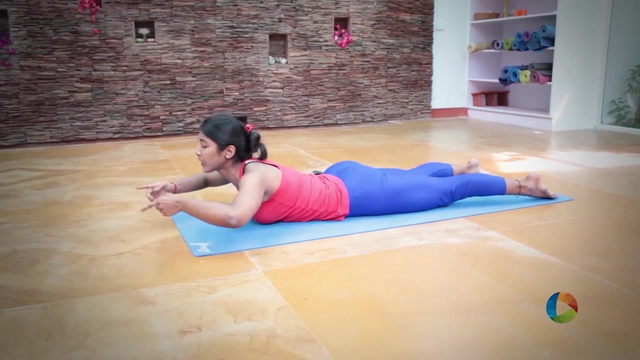 inhale. lift the left arm up, exhale down. release the legs and repeat on the other side. Lie on your abdomen, open your legs out slightly. place your palms in between your chest and your pelvic bone. Now inhale and then come up. Feel somebody is pulling your neck. lengthen. 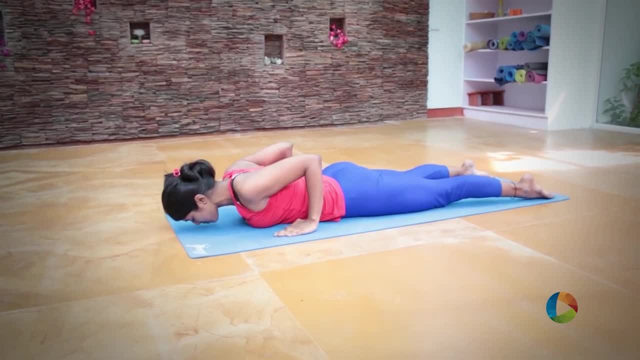 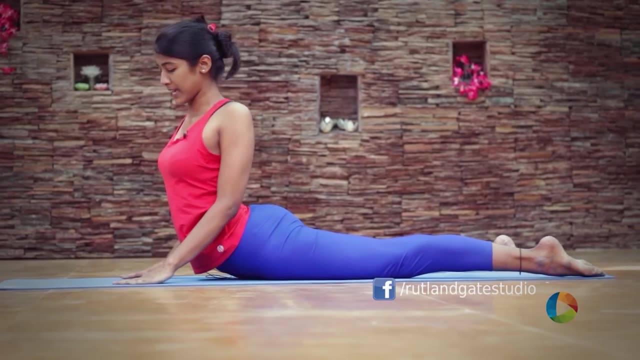 your neck and then come all the way up towards the ceiling and then arch back, Inhale. come up, arch back, Push your pelvic bone down, Allow your pelvic bones to protrude towards the mat and then stretch your lower abdomen. Don't bend your elbows, Press the elbows and 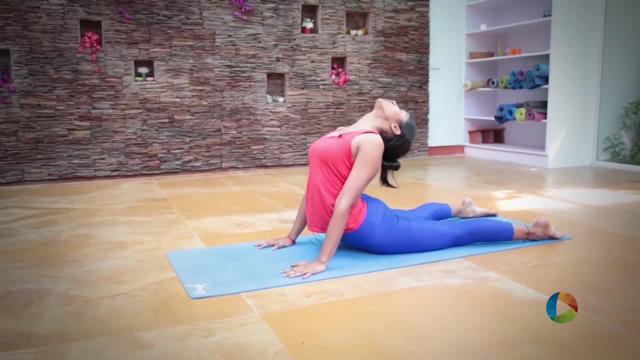 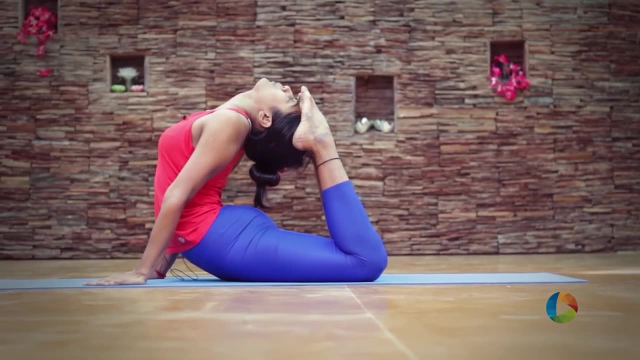 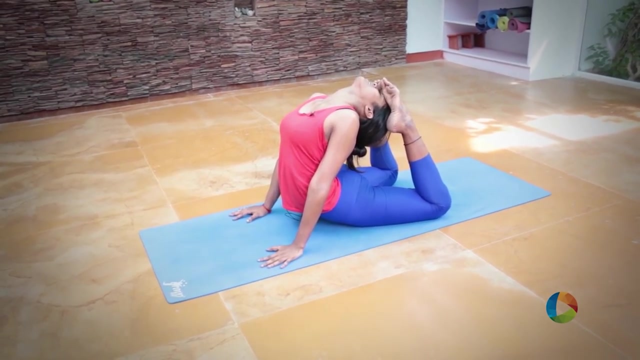 you don't shrug your shoulders. Open your shoulders out, arch back, drop your neck down and then lift your legs up. Nice stretch for your quadriceps. This is called Kapotasana. Keep pushing your pelvic bone down, tighten your butt muscles. Breathe, mind breathe. 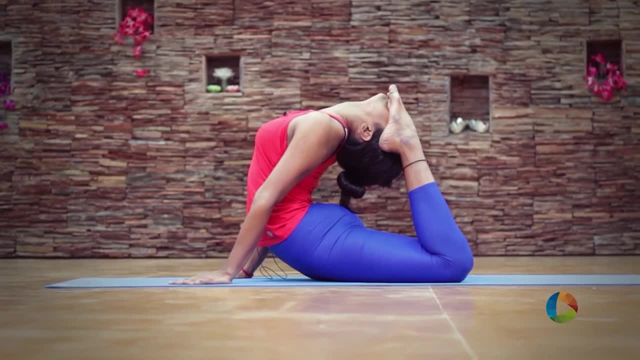 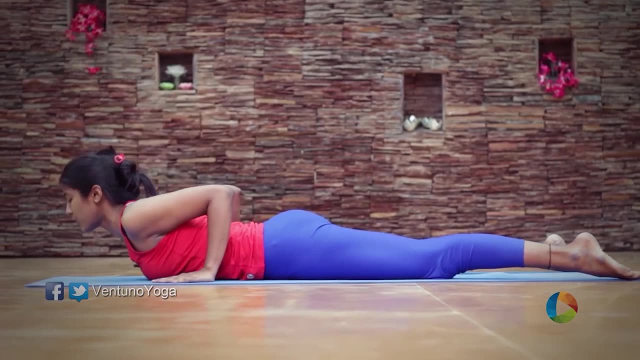 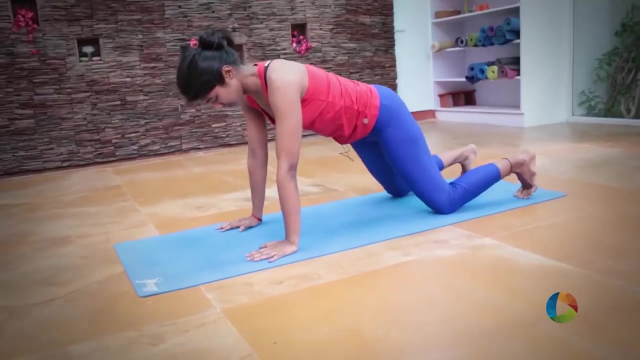 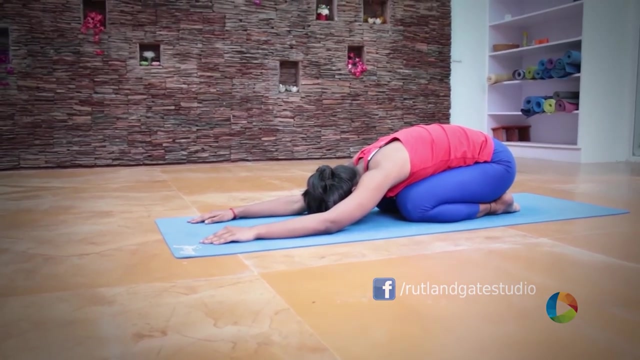 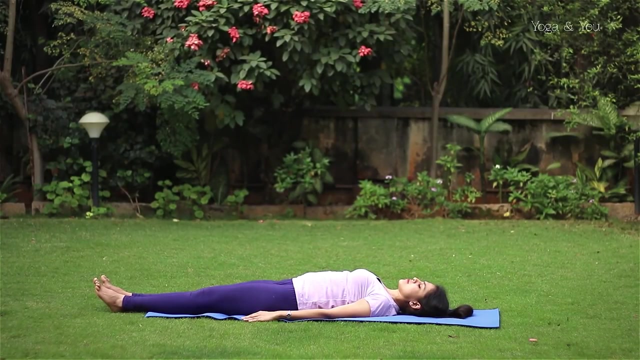 Inhale down And then relax, And then come to Shishangasana. Stay here for five to six seconds. Halasana From the supine position. raise your legs 90 degrees. Inhale, lift the hips. 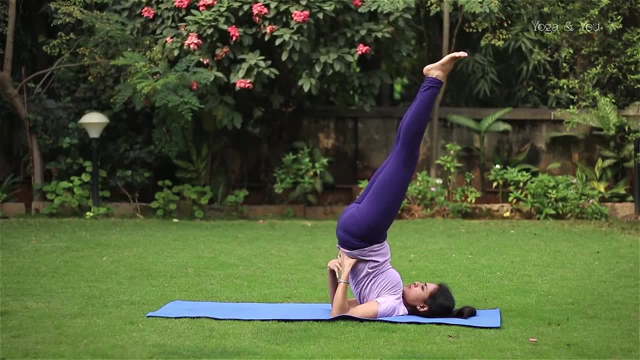 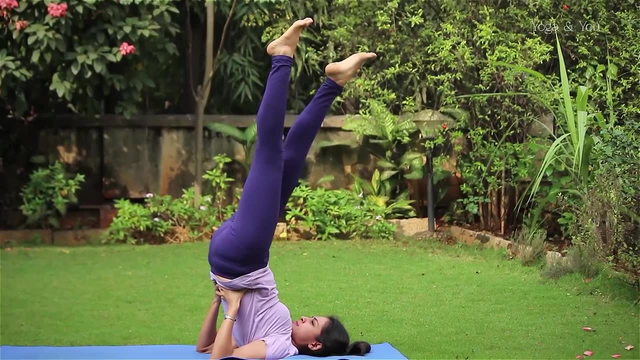 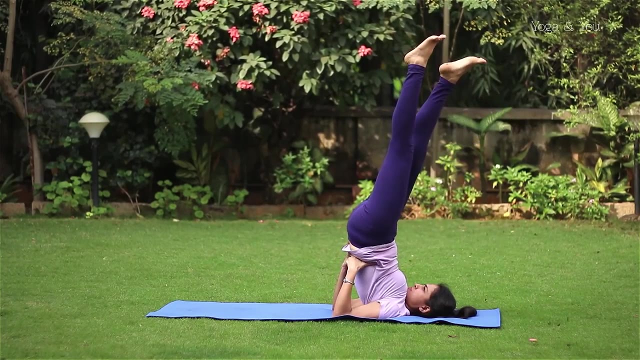 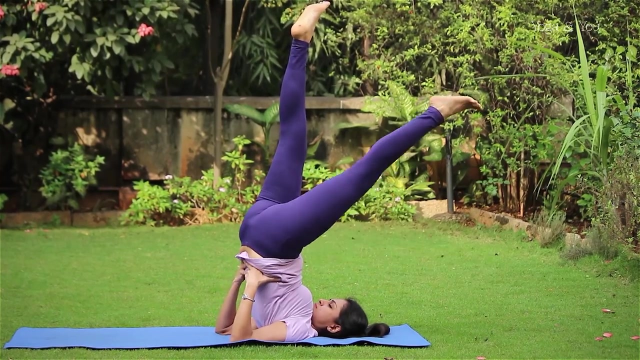 up and support your back. Come into Sarvangasana Now. slowly. bring your right leg down behind the head onto the floor, keeping the knees straight. Inhale up And exhale. bring the left leg down behind the head onto the floor. Inhale up, Keeping the back supported slowly. 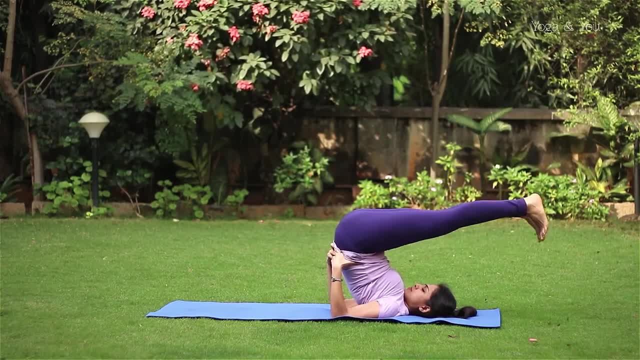 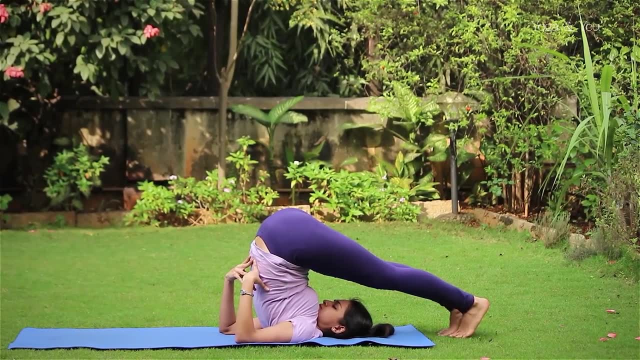 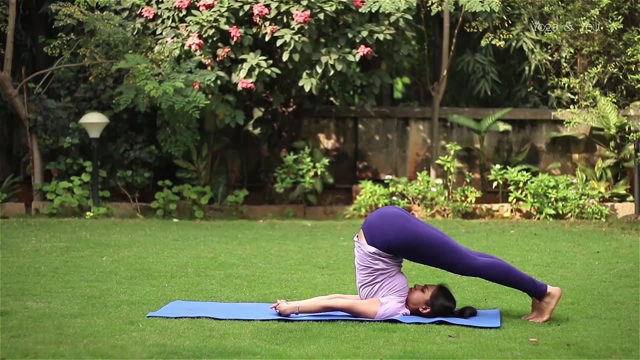 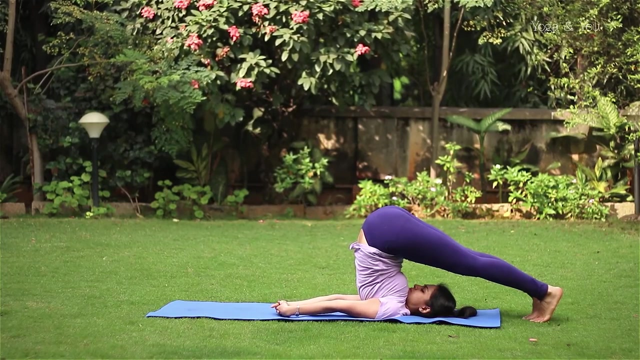 with control. bring both legs down behind the head onto the floor, keeping the knees straight. Keep the back supported till your feet touch the floor. Walk your toes towards the head. Release the hands. Interlock the fingers behind your back To release the asana. first release your hands. Place your palms down on the mat. Raise the. 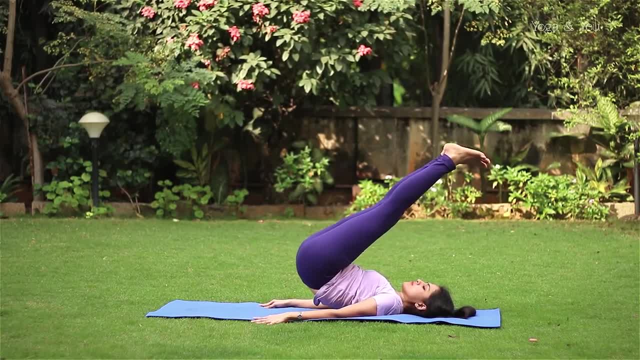 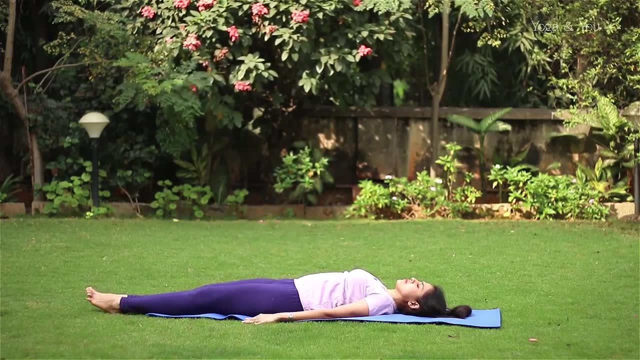 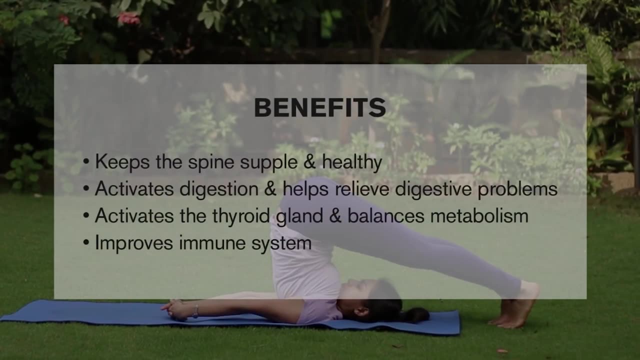 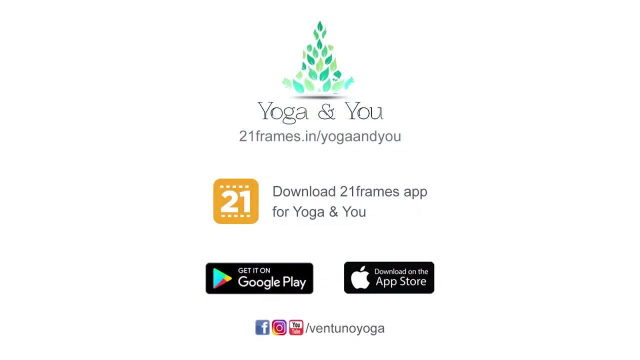 legs 45 degrees above the head. Roll out vertebra by vertebra, Slowly, with control. bring your legs down to the mat, Inhale up And exhale. bring your legs down behind the head, onto the floor, keeping. the knees straight.